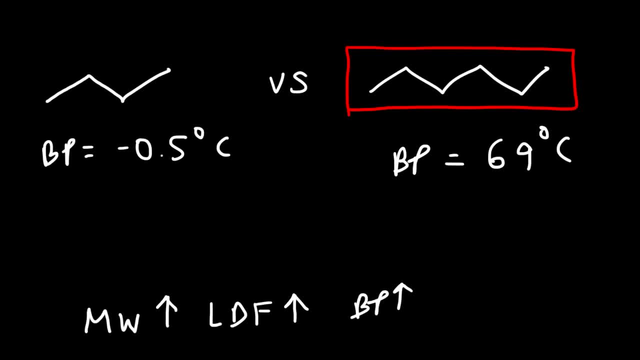 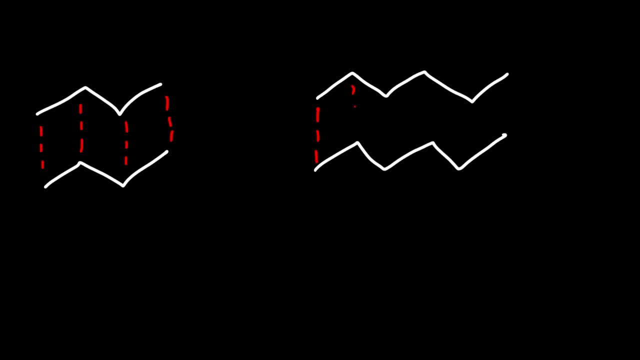 And this will increase the boiling point of hexane. So this is butane, And let's draw another butane molecule next. So we have dispersion forces that can keep these two molecules together. Now the same is true in hexane. Hexane will have more London dispersion interactions than butane. Because hexane has six carbons and butane only has four carbons, And so whenever you're dealing with nonpolar molecules, as you increase the number of atoms, the molar mass will increase or the molecular weight will go up. 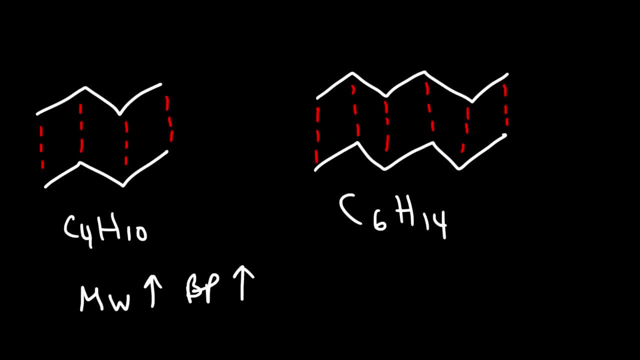 and this will increase the boiling point of that compound. So, for example, let's say, if we have an alcohol, one butanol, and we compare it to one hexanol, Which one is going to have the higher boiling point? It's going to be this molecule because it's bigger. 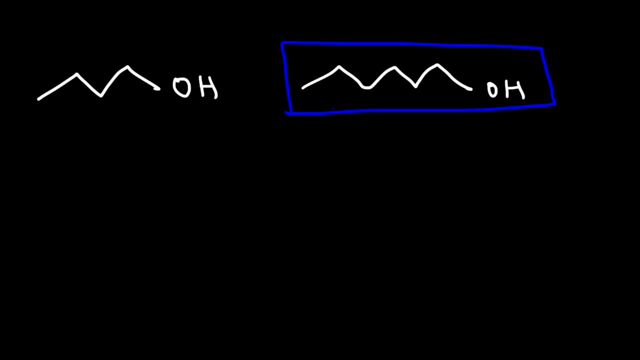 And so bigger molecules with more atoms, they will always have a higher boiling point. Now what about these two examples, Acetaldehyde and ethane? Which one will have a higher boiling point? So feel free to pause the video if you want to think about it. 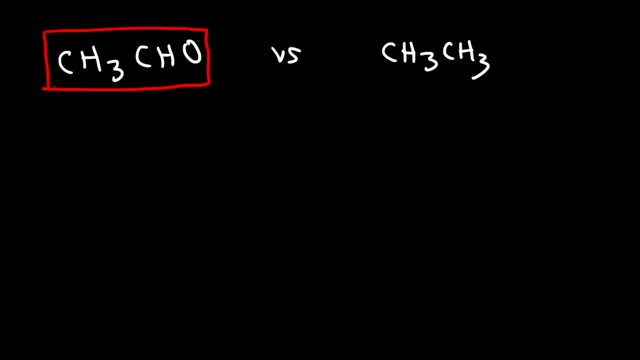 The answer is going to be acetaldehyde. Acetaldehyde has a boiling point of about 20 degrees Celsius, and ethanol is going to have a boiling point of about 20 degrees Celsius, And ethane has a boiling point of negative 89 degrees Celsius. 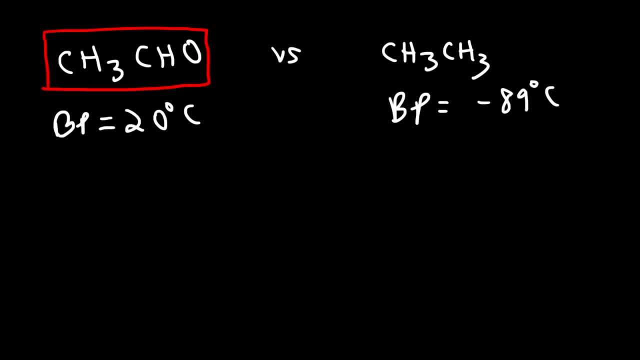 Whenever you have a hydrocarbon that contains only carbon and hydrogen atoms, that molecule is nonpolar, But because of the aldehyde functional group, this molecule is polar And with everything else being the same, let's say, if we have similar molar masses between the two molecules, 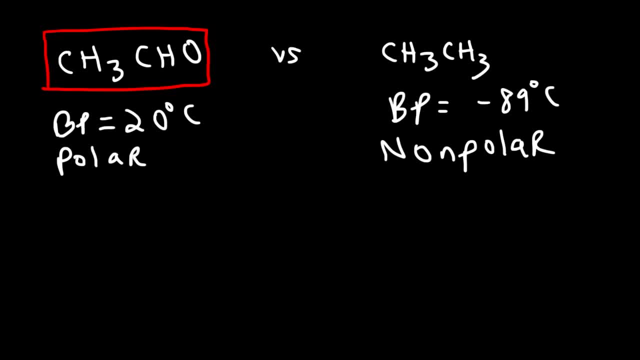 a polar molecule will usually have a higher boiling point than a nonpolar molecule. Polar molecules have dipole-dipole interactions in addition to London dispersion forces, whereas a nonpolar molecule only have dispersion forces, And dipole interactions are a lot stronger than dispersion forces. 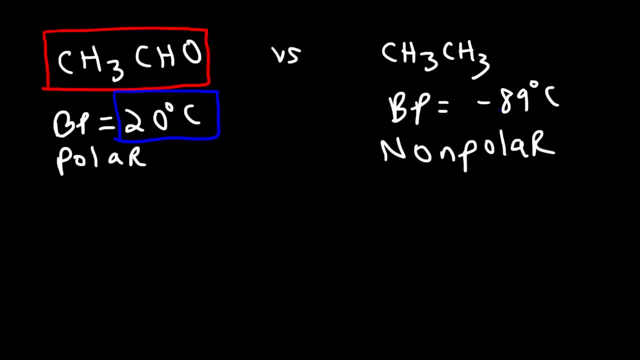 And so you can see the huge difference in boiling point between these two molecules. Now let's show the dipole interactions between two acetaldehydes and ethanol. So let's look at the dipole interactions between two acetaldehydes. Oxygen is more electronegative than carbon. 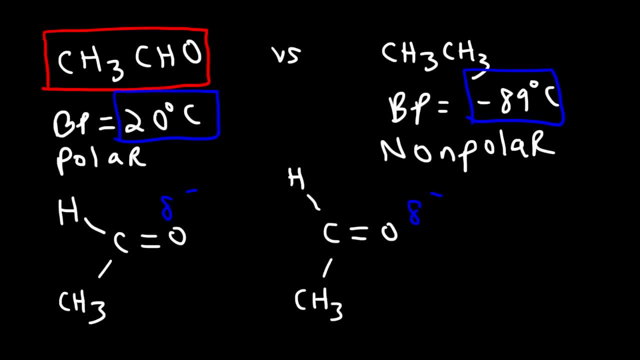 So in the CO bond oxygen is going to bear the partial negative charge and carbon will bear the partial positive charge. So the oxygen of one of these molecules is attracted to the carbon of the other because this one has a negative partial charge. 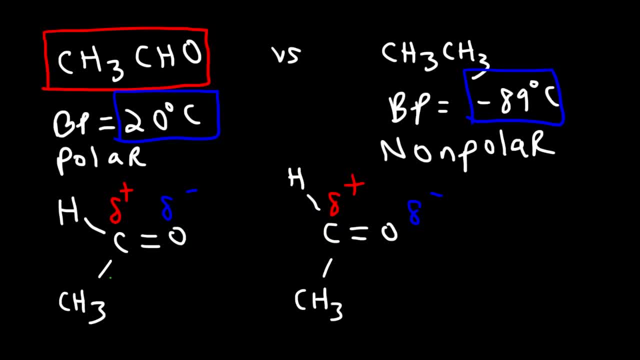 and this one has a positive partial charge. And so this one has a negative partial charge and this one has a positive partial charge. So this is going to be a force of attraction that will connect these two molecules together, And so that interaction is known as a dipole-dipole interaction. 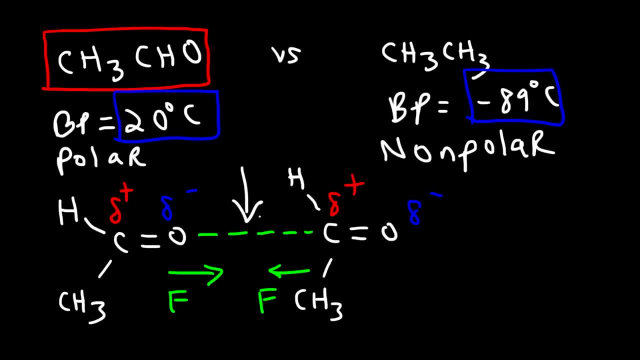 It's between two molecules and it's a strong interaction compared to dispersion forces. In order to boil this substance, you need to separate the molecules from the liquid state and move them apart so they can enter the gas state. To do that, you have to add heat to break this interaction that holds them together. 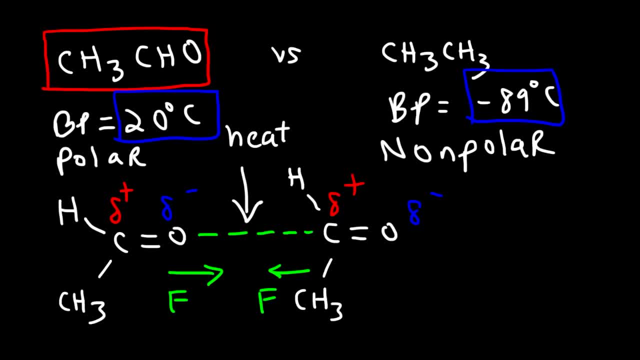 And so the stronger the interaction, the more thermal energy you've got to put in to break those dipole-dipole interactions, thus increasing the boiling point of the substance. So a molecule with a high boiling point tells you that you need more thermal energy to break the intermolecular forces. 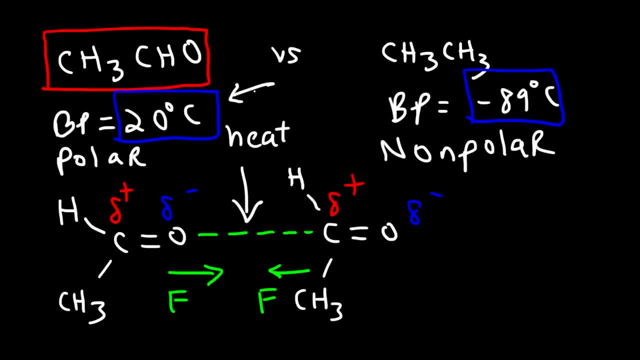 that hold those molecules together in the liquid state, Because in the case of ethane, the boiling point is so low. that tells us that the intermolecular forces that hold ethane molecules together is very, very weak. It doesn't require much thermal energy. 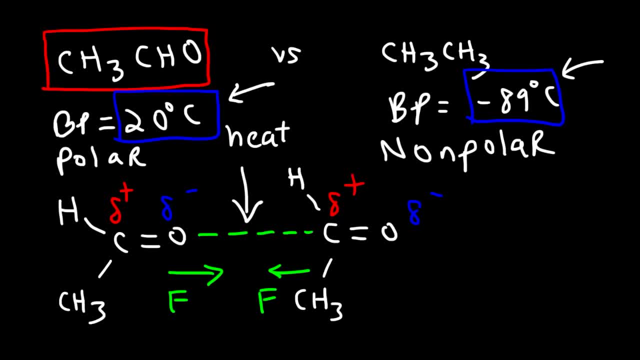 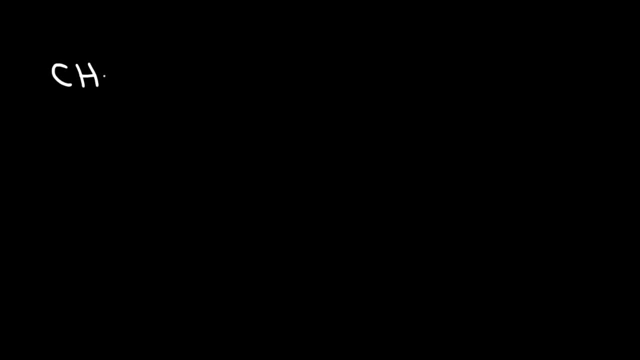 to separate one ethane molecule from another because it has weak LDF forces. Now let's compare acetaldehyde with ethanol. Acetaldehyde is also called ethanol with an AL, and on the right we have ethanol with an OL. Which of these two molecules will have a higher boiling point? 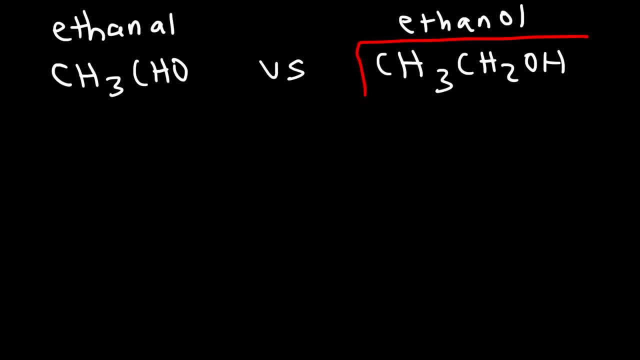 It turns out that ethanol has a higher boiling point than ethanol or acetaldehyde. The boiling point of ethanol is 78 degrees Celsius, and for acetaldehyde we saw that it was 20. So why is it so much higher, when in fact both of these molecules are polar? 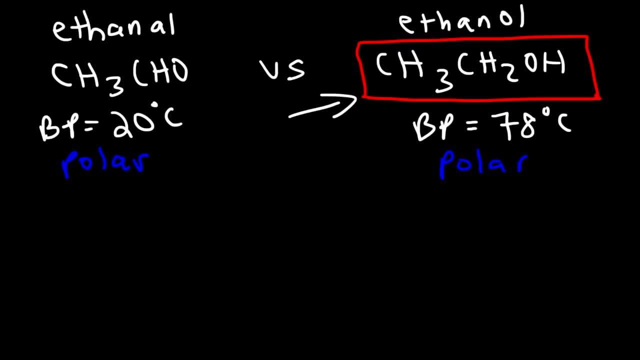 They both contain dipole-dipole interactions. Ethanol, however, contains a special type of dipole-dipole interactions known as hydrogen bonds. Whenever hydrogen is directly attached to nitrogen oxygen or fluorine, you're going to have hydrogen bonds. 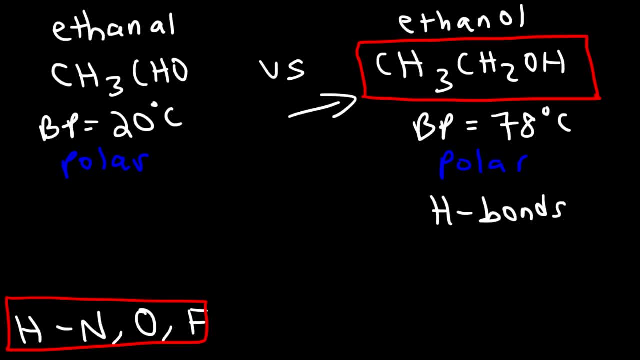 A hydrogen bond is a stronger type of intermolecular force than a dipole-dipole interaction, And so that's why we can see that ethanol has a higher boiling point than acetaldehyde. So if you look at acetaldehyde, if you draw it, 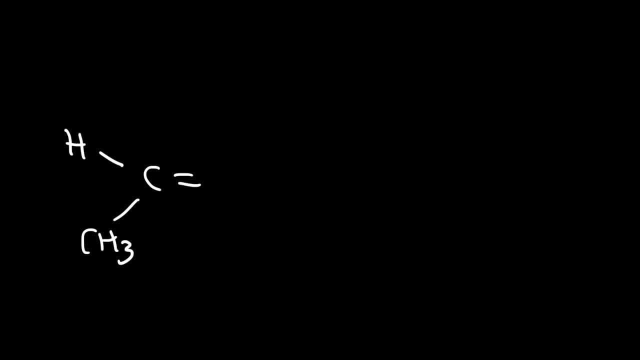 you can see that the oxygen is not directly attached to the hydrogen. So that's why there's no hydrogen bonds in this molecule or between molecules of acetaldehyde. The O has to be directly attached to the H. Now, when you see it this way, 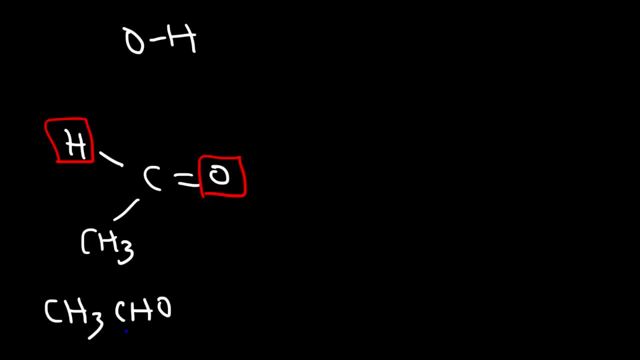 it may appear as if H is directly attached to O, but it's not when you draw it out, So watch out for that. Now, in the case of ethanol, if we draw it, I'm going to use a line structure to represent it. 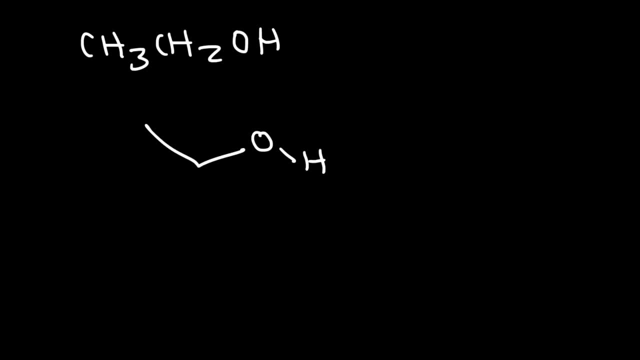 The oxygen is directly attached to the hydrogen. The oxygen has a negative partial charge and the hydrogen has a positive partial charge. So let's put this next to another ethanol molecule. So, like the dipole-dipole interaction, opposite charges will attract. So the partially positive hydrogen atom is: 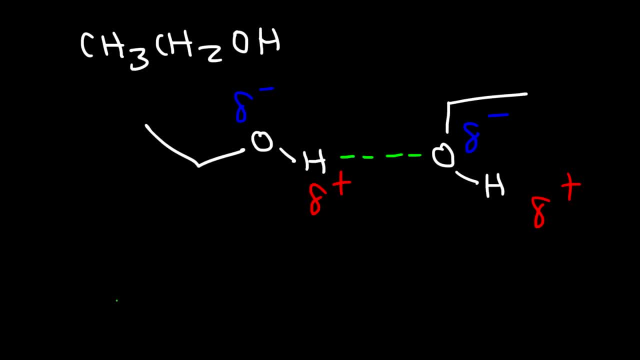 going to be attracted to the oxygen with a negative partial charge, And so that interaction is the H bond. So hydrogen bonds exist between two separate molecules as opposed to within a single molecule, And so these H bonds, they keep the ethanol molecules together in a liquid state, And so that's why it. 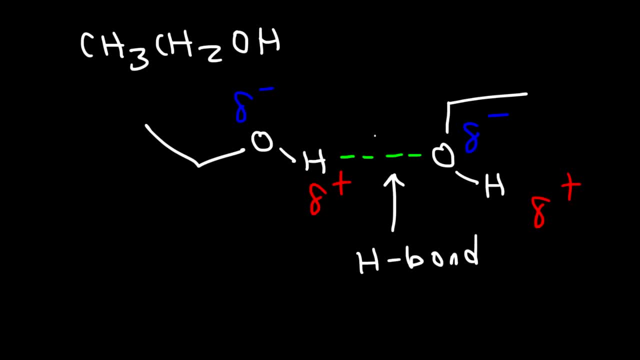 requires so much energy to separate these ethanol molecules, to put it in the gas state, And that's why the boiling point is so high. So that's why the boiling point is so high, Because hydrogen bonds are stronger than dipole-dipole interactions. 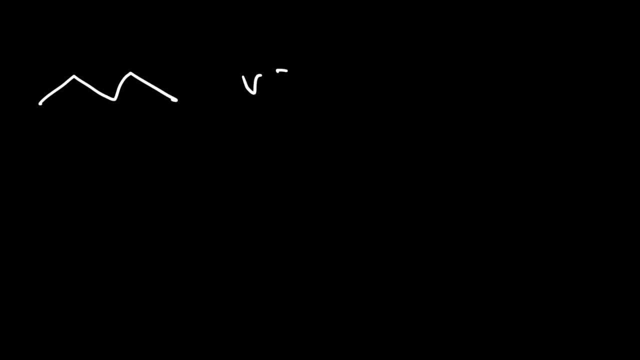 Now let's compare pentane with neopentane. Which of these two molecules will have a higher boiling point? The answer is going to be pentane. The question is why Pentane has a boiling point of about 36 Celsius and for neopentane it's about 9.5.. So clearly, for pentane it's higher And it 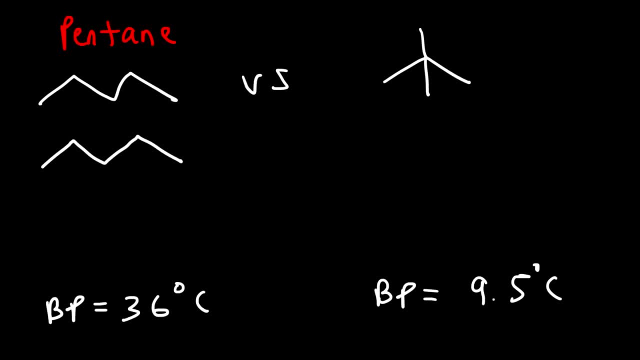 has to do with the structure of the molecules. In pentane, the contact area between two pentane molecules is greater than that in neopentane. So if you try to stack one neopentane molecule next to another, notice that the interaction will. 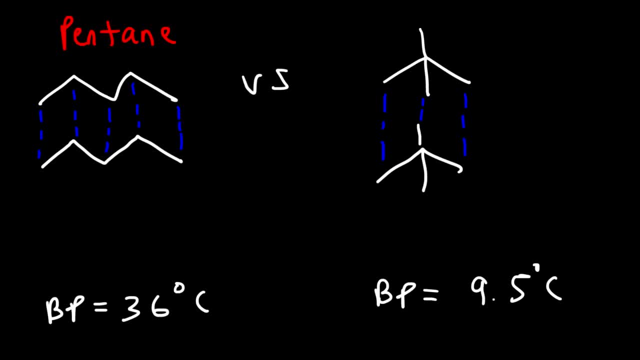 be a lot less, And it's due to branching. Because this molecule is highly branched, the contact area is reduced And so anytime you have branching, the boiling point goes down Because there's going to be less London dispersion forces between the nonpolar. molecules, And so that decreases the boiling point. So straight-chain alkanes have a higher boiling point than branch alkanes. Now make sure that the number of carbon atoms is the same, So in both cases we have the same molecular weight due to the same formula. 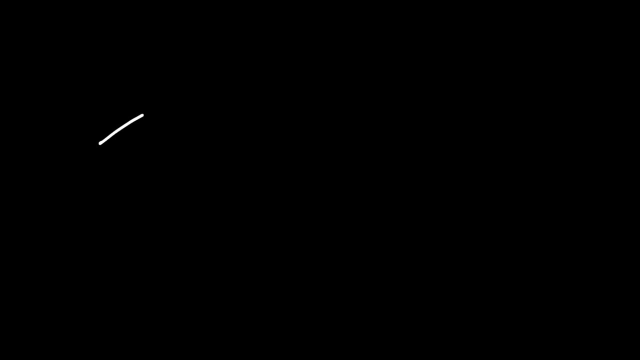 C5H12.. Now let's compare two alkyl halides, ethyl chloride and ethyl bromide. Which one is going to have a higher boiling point? The answer is going to be ethyl bromide. The bromine atom is bigger than the chlorine atom And, as a result, 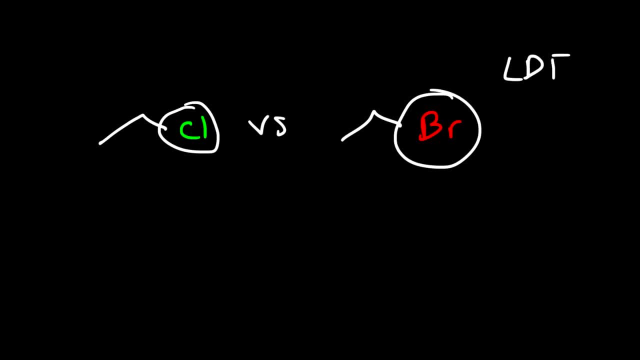 it's going to have more London dispersion forces. Because it's electron cloud, it's going to be more polarizable And so, because it's bigger, it has more contact area And so when you're dealing with bigger atoms, they will have a. 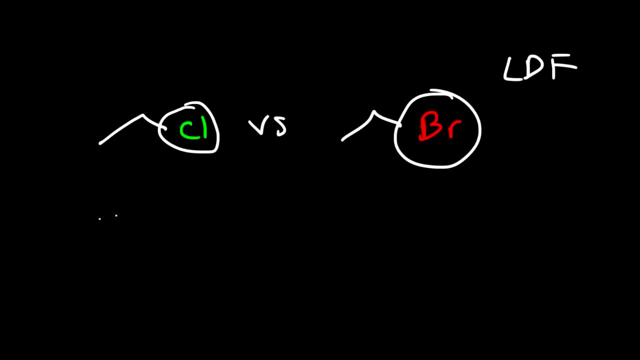 higher boiling point compared to smaller atoms. The boiling point for ethyl chloride it's about 12.. And for ethyl bromide it's 38.. For ethyl fluoride it's going to be the lowest because fluorine is the smallest. 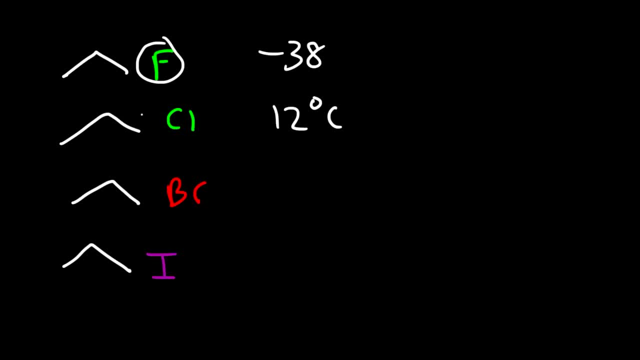 in the group We said for ethyl chloride the boiling point is 12.. Chlorine is a little bit bigger than fluorine, And then bromine is bigger than chlorine And iodine is a lot bigger than bromine. And so, as you can see, as the size of the 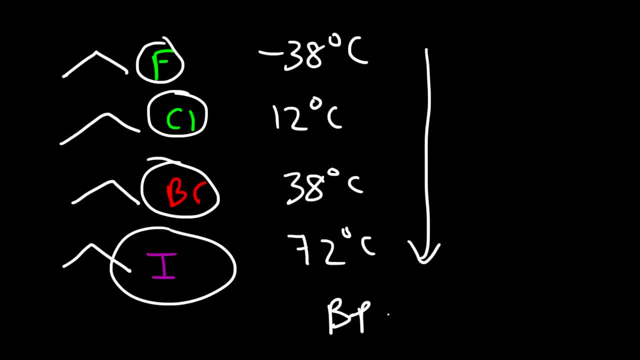 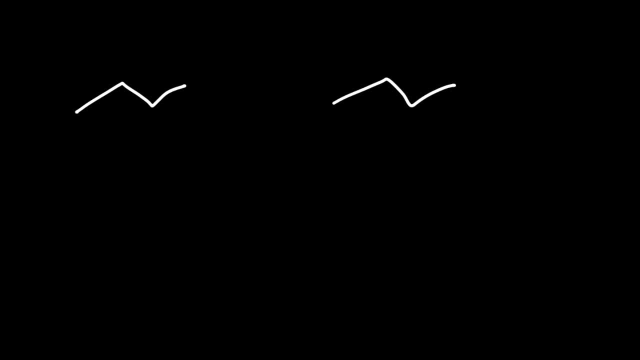 halogens increases, the boiling point will increase. Now let's compare the boiling point of an alcohol with a primary amine. Which one is going to have the higher boiling point? Now we know they both contain hydrogen bonds, Because anytime H is directly attached to N. 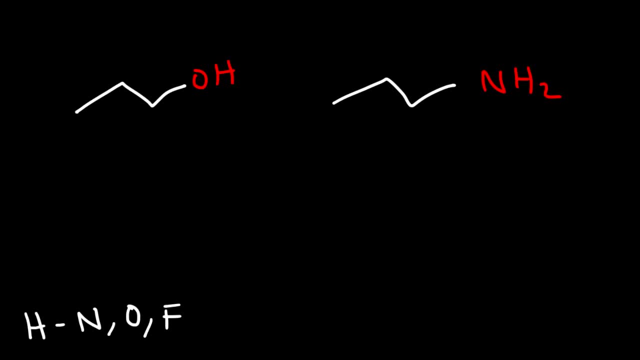 or F, you have H bonds, And they both contain the same number of carbon atoms, So the molecular weight between these two molecules are very similar. Now the OH bond is more polar than the NH bond. The electronegativity for nitrogen is: 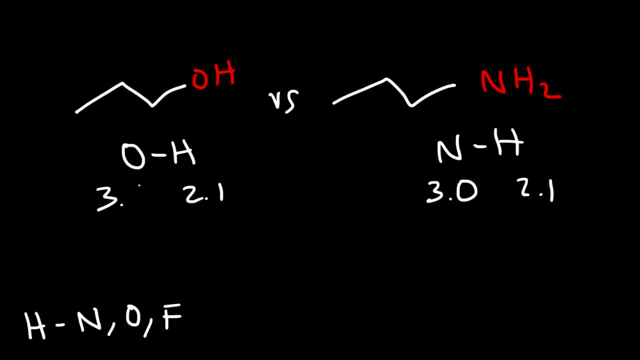 3.0, and for hydrogen is 2.1.. But for oxygen is 3.5.. So the EN difference between the two atoms: in the case of the OH bond it's 1.4.. And the electronegativity difference for the NH bond is 0.9.. So because oxygen is more electronegative, 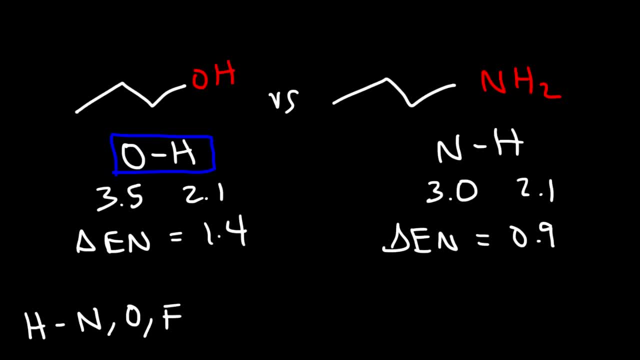 than nitrogen. the OH bond is more polar than the NH bond, And so it turns out that a primary alcohol has a higher boiling point than a primary amine. In fact, the boiling point for this primary alcohol is about 97 degrees Celsius, And for the primary amine it's 48 degrees Celsius. So 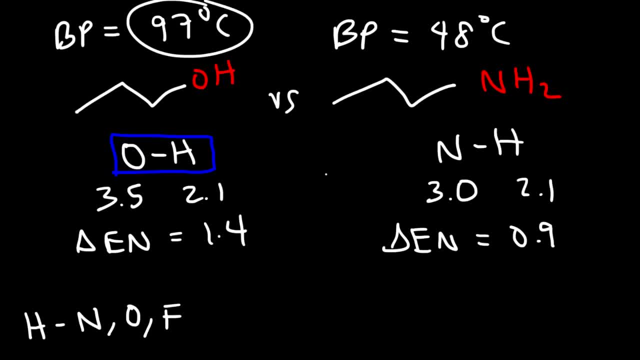 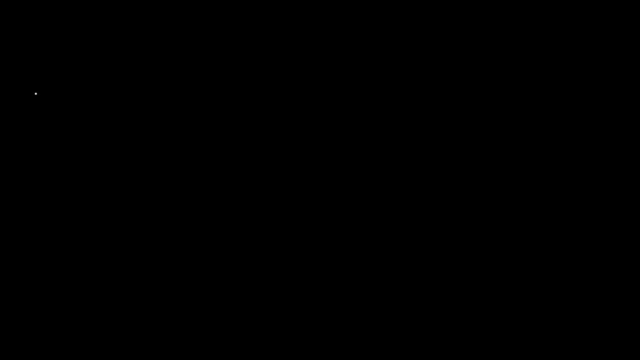 97 is a lot higher than 48. So alcohols have higher boiling points than their correspondent amines. Now let's try this example. Let's say if we have a primary amine, a secondary amine and also a tertiary amine. 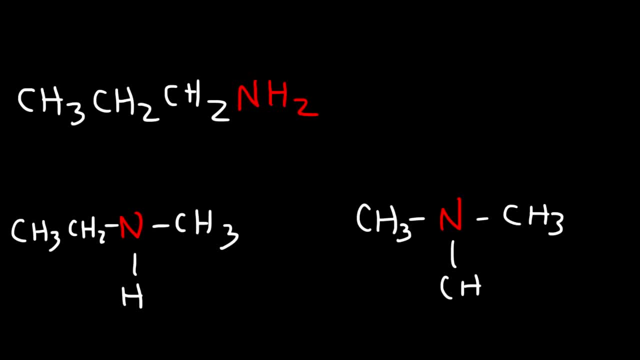 So which of these amines will have the highest boiling point? What would you say? Is it the primary amine, The secondary amine Or the tertiary amine? So we know that the boiling point of the propyl amine it's 48 degrees Celsius. Now for the 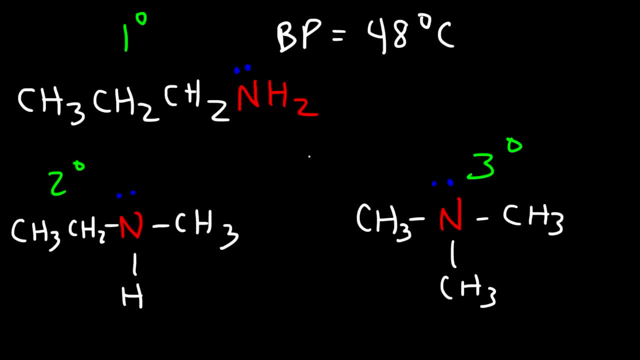 secondary amine. I had to look this up. I found some varying numbers, but most of the answers were around 36, 37 degrees Celsius, And for trimethylamine, the boiling point that I found was approximately three degrees Celsius. Now it's understandable why this one is the lowest of the three, because nitrogen is not directly attached to hydrogen. 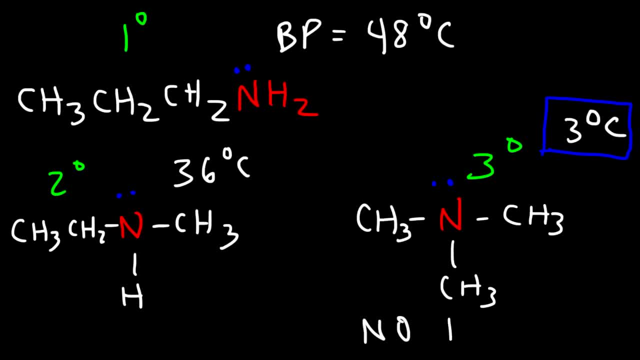 So for a tertiary amine, it has no hydrogen bonds. So that's why the boiling point for the tertiary amine is significantly lower than the other two amines. Now, looking at the primary amine versus the secondary mean, the boiling point for 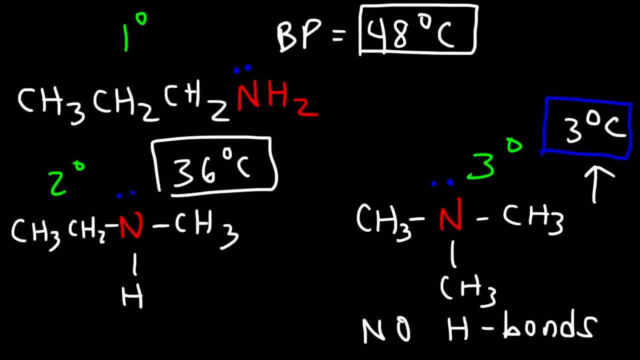 the primary amine is slightly higher than the secondary secondary amine. They both contain hydrogen bonds, but the NH2 molecule has two hydrogens attached to the nitrogen compared to the NH molecule in the secondary amine. But for the most part primary amines have higher boiling. 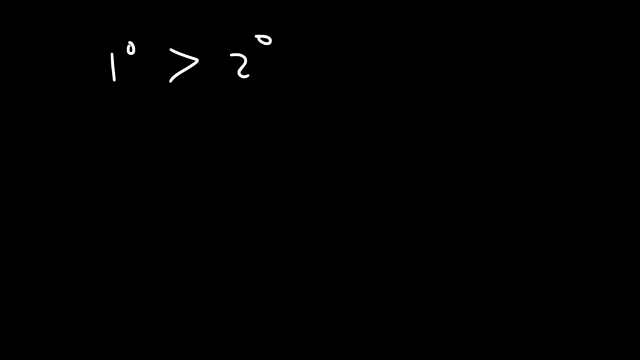 points than secondary amines, and secondary amines have higher boiling points than tertiary amines. So here you have an NH2 group. So you got two NH bonds and here there's only one NH bond, and for this one there's no NH bond. So